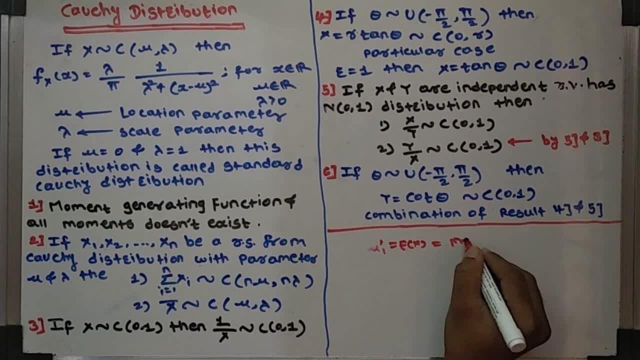 of x, which implies that mean which is mean does not exist, and variance of x is also moment which is mu1. that is equal to expectation of x minus expectation of x is also moment which is does not exist. Therefore, variance is also does not exist for this distribution. 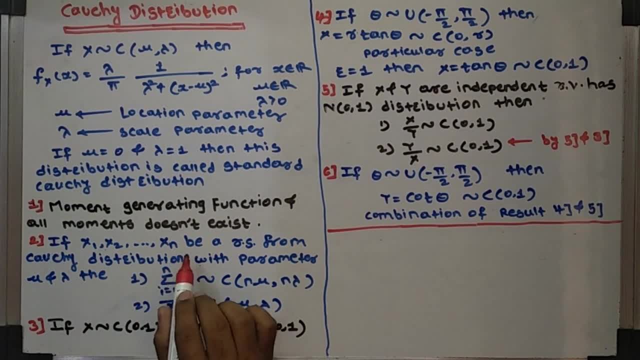 Second result is: if x1 comma, x2 comma, dash, dash, xn be a random sample from Cauchy distribution with parameter mu and lambda, then summation of xi follows Cauchy distribution with parameter n, mu, comma, n, lambda, That is, xi follows iid with Cauchy distribution with parameter mu. 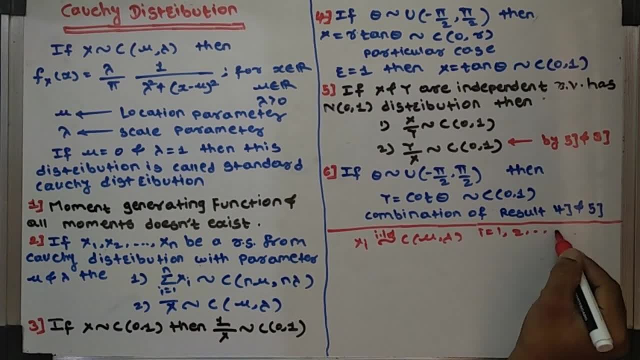 comma lambda For i equal to 1 to comma dash dash n. then summation of xi follows Cauchy distribution with parameter n, mu, comma n, lambda. See this property is look similar to the additive property but in this property parameter first is mu for x1, x2, comma xn are same and second parameter. 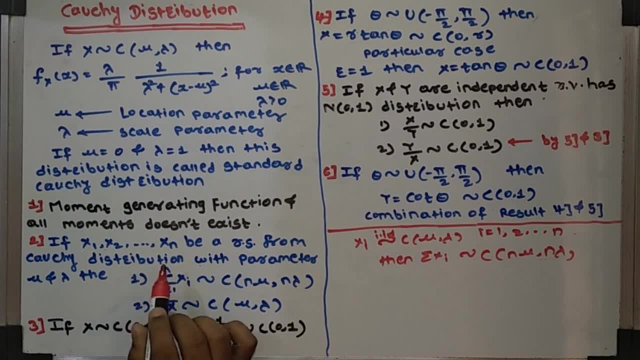 is lambda. also same for x1, x2 comma xn. So also this result implies that mu is equal to 0 if x equals to 1.. And third result implies that x bar follows Cauchy distribution with parameter mu comma lambda. 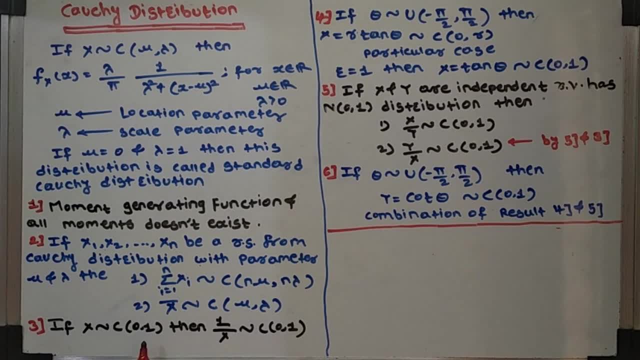 Here distribution of xi and x bar are same, which is Cauchy distribution with parameter mu comma lambda. Third result is: if x follows Cauchy distribution with parameter 0 comma 1, that is x follows standard Cauchy distribution, Then 1 upon x also follows. 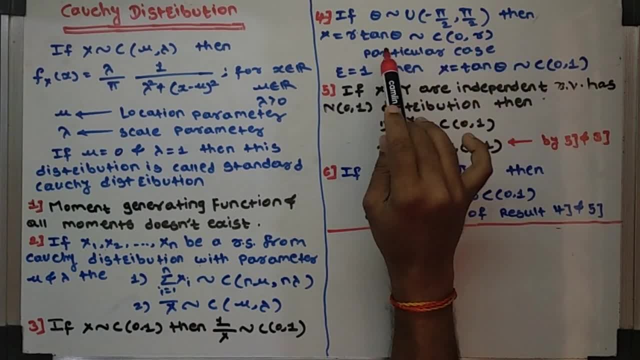 uniform minus pi by 2 to pi by 2, then x equal to r tan theta. follows Cauchy distribution with 0 comma r, here r is from. here this has a particular case: if r equal to 1, then x equal to r tan theta. 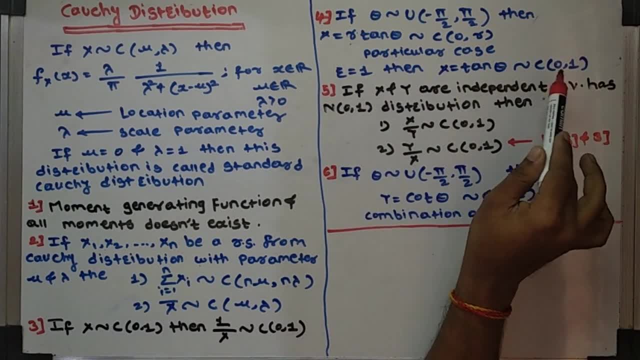 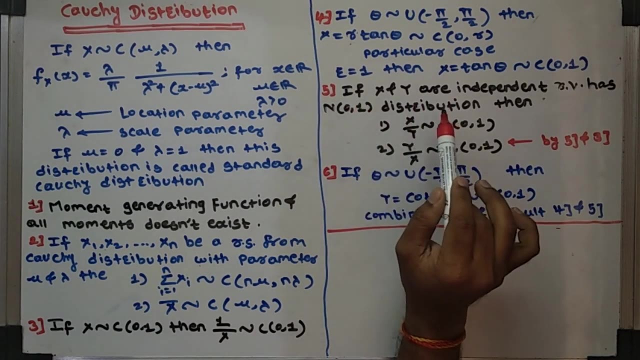 means here we put r equal to 1, so tan theta follows Cauchy 0 comma 1. that is standard Cauchy distribution. that is theta follows uniform minus pi by 2 to pi by 2. then tan theta follows standard Cauchy distribution. fifth result is: if x and y are independent random variable has normal 0 comma 1. 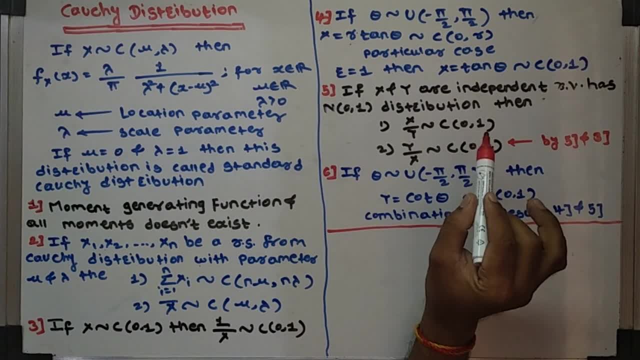 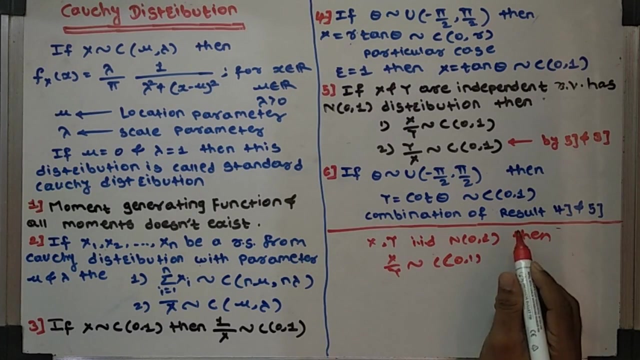 distribution, then x upon y follows Cauchy distribution with 0 comma 1, that is here x comma y are iid from normal 0 comma 1, then its ratio that is x upon y. follows Cauchy distribution with parameter 0 comma 1, that is x comma y from standard normal, then its ratio is also follows: 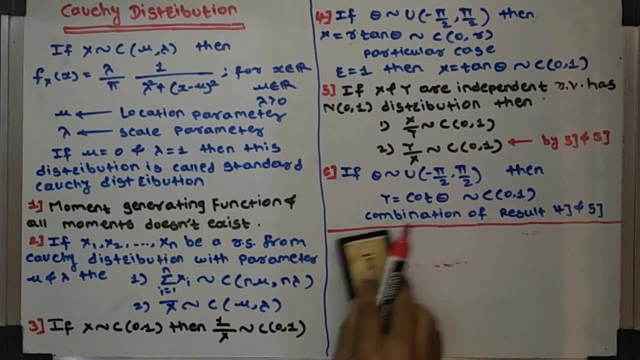 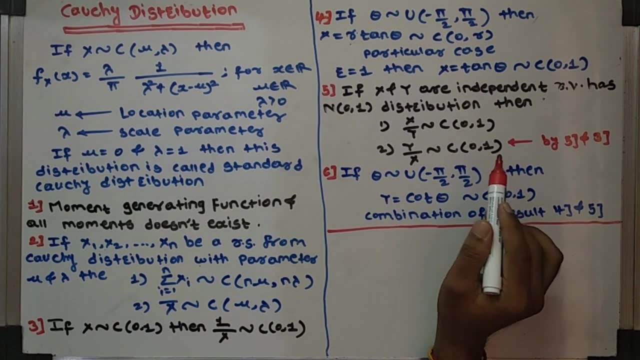 standard Cauchy distribution. here we see in second part: y upon x. also follow standard Cauchy 0 comma 1. we see in fifth result: x comma 1, y follows normal with 0,1. here x and y are iid. then x upon y follows cos 0,1. here we. 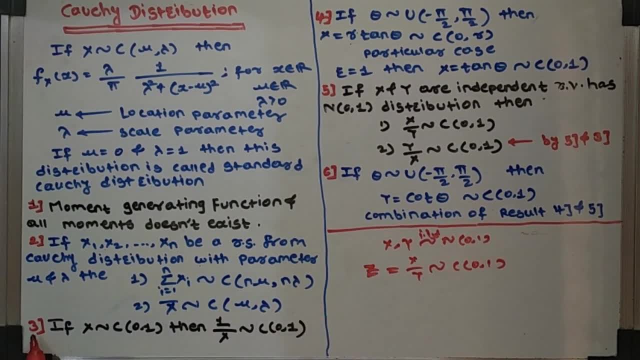 let z equal to x upon y. so from third result: x follows cos 0,1. here z follows cos 0,1. then 1 upon x means 1 upon z. that is equal to one upon x upon y, because z is equal to x upon. 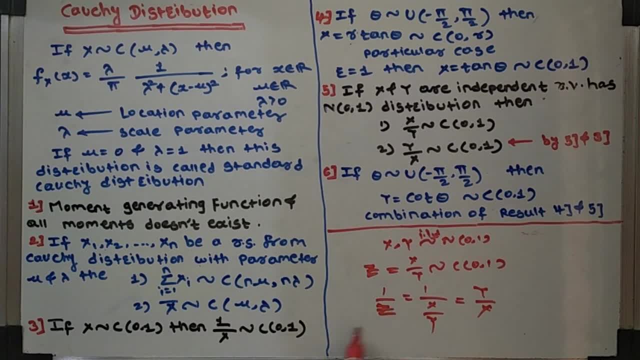 y, that is equal to y upon x. by this result 1 upon z follows cos 0,1. therefore y upon x follow cos 0,1. so we take ratio of two of any. then this also goes standard cos distribution. so sixth result is: if theta follows uniform minus 5 by 2.. 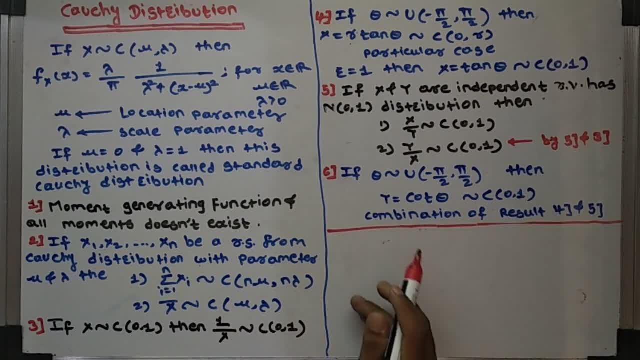 2. 2. pi by 2, then y equal to cot. theta follows standard Cauchy distribution. this result is also combination of fourth result and third result. here see in sixth result. theta follows uniform minus pi by 2 to pi by 2 by result 4. here we see in particular case r, equal to